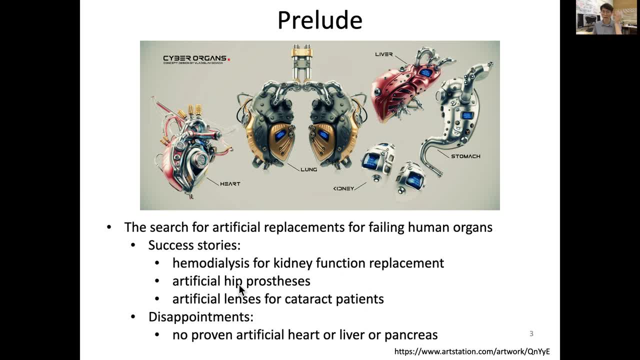 And also for people who have a problem in the eye lens. there are artificial lenses for cataract patients. Cataract is the symptom that the lens become opaque so that the patient cannot see. My parents also have this cataract surgery, which is one of the most common surgeries in our country. 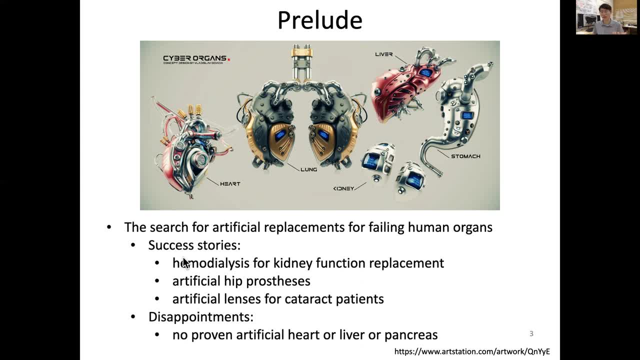 However, these are a good success stories, but are limited. You can see, these are relatively simple aspects of biomaterial, But this point is, there are no proven artificial hearts, artificial liver or artificial pancreas, So which poses a great challenge at the same time. 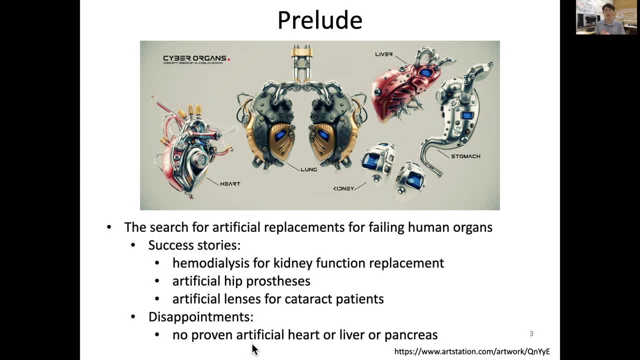 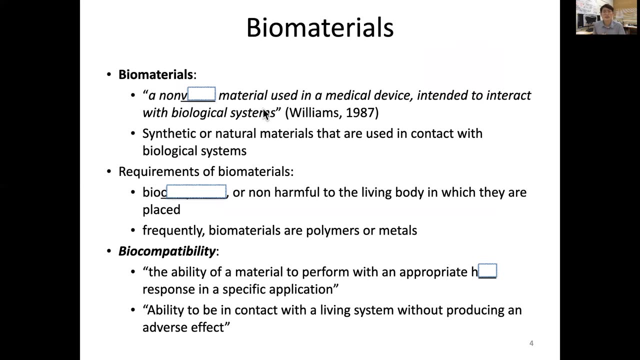 an opportunity for biomedical engineers like us to develop these more sophisticated organs which potentially can benefit many, many people who have problems in their organ function. So let's first see what is biomaterials. There are some historic definitions. I want to introduce A non-viable material used in a medical device which is intended to interact with our biological 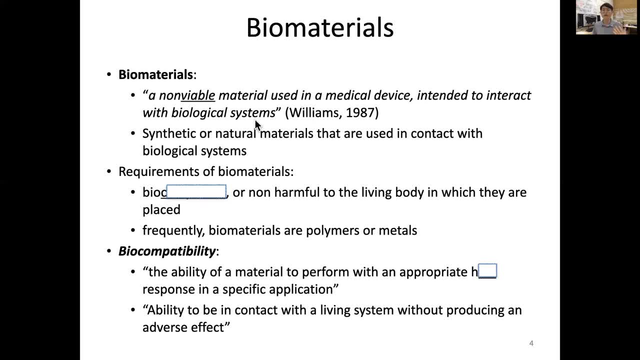 systems. Another way of looking at it is synthetic or natural materials that are used in contact with biological systems. So for the biomaterial, there are requirements for biomaterial because that is in contact with our biological system, So it has to be non-harmful to the living body in which they are placed. 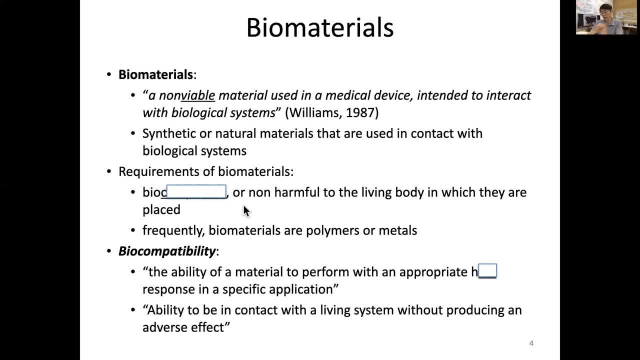 So that we call as whether it's compatible or not. So that's called biocompatibility. So frequently biomaterials are polymers or metals, So polymers are more like soft aspects of replacement and hard aspects such as bone, and there are metal. 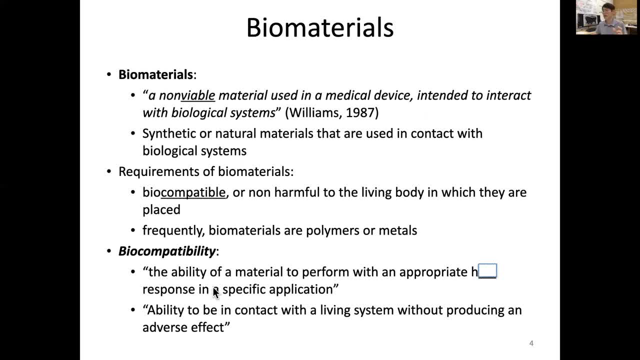 So biocompatibility is the ability of a material to perform with an appropriate host response in a specific application. Host response means our body's natural response, For example, like immune system against some foreign body, foreign material Which is coming into our body, And biocompatibility is the ability to be in contact with. 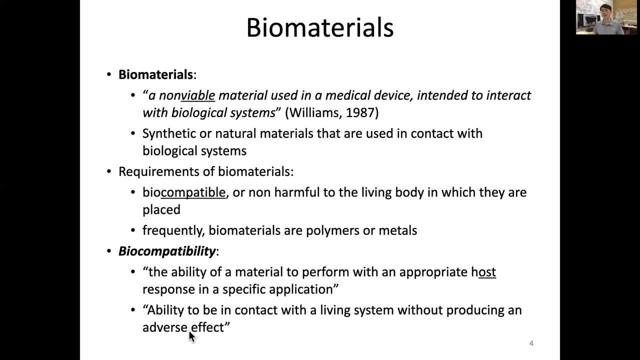 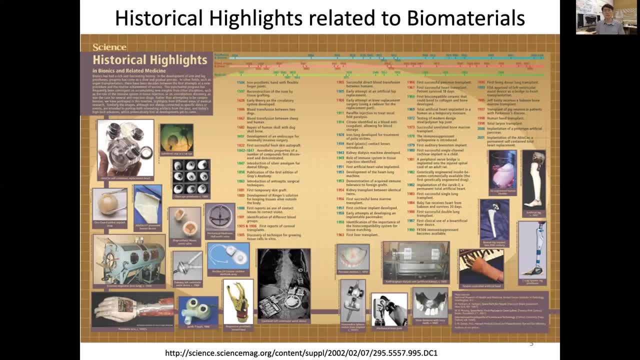 a living system without producing an adverse effect. So I want to discuss about some history. So there are pretty good review, historical highlights, which is related to biomaterial, Especially bionics and related medicine. You can see it starts from even like over 500 years ago until today. 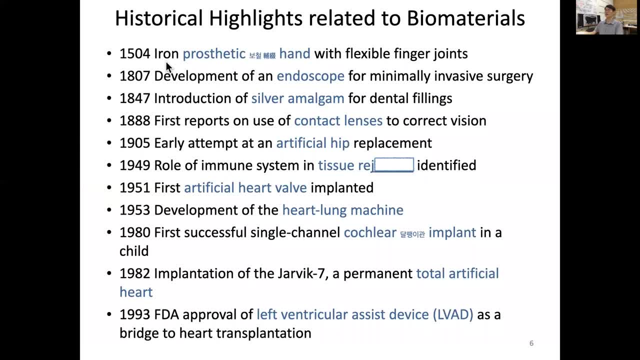 So let me go through a little bit of these histories. So about 500 years ago there were iron prosthetic hands, So for those who lost hand with a flexible finger joint was found. And about 200 years ago, development of endoscope for minimally. 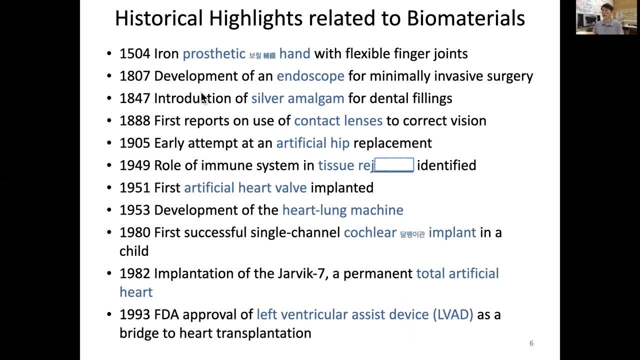 invasive surgery, We developed an endoscopy And, about more than 75 years ago, introduction of silver amalgam for dental fillings. In 1888, first report of contact lens to correct vision. And 1905, early attempt of an artificial hip replacement for those who have a problem in the hip. 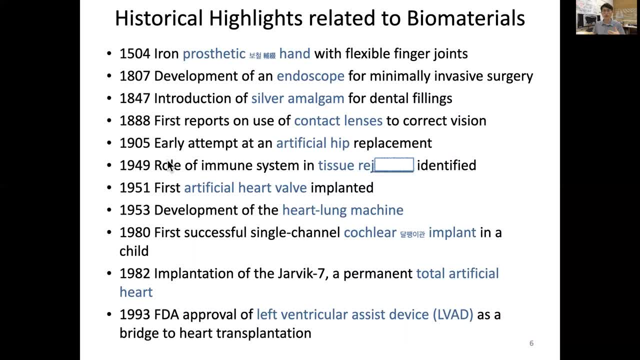 joints And only after quite recent, about 1949,, the role of immune system in tissue rejection is identified. What do we mean by tissue rejection? If there's an artificial biomaterial getting into the tissue, then our immune system will sometimes reject. Or when we do a transplantation of an organ from 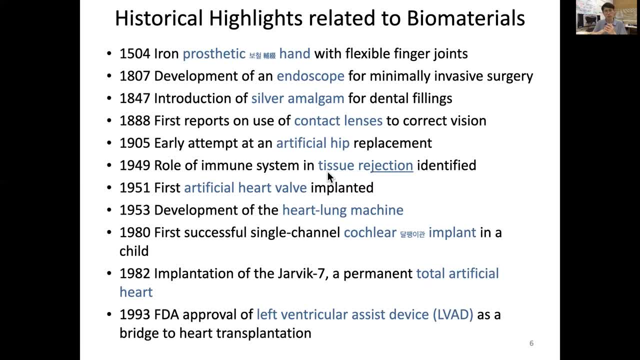 other person to other person we can see that the tissue is rejected. So we can see that the tissue is being translated to their own organ And when we call it a host then the host system will recognize it as a foreign and try to reject that organ. That is a big problem still in organ transplantation. 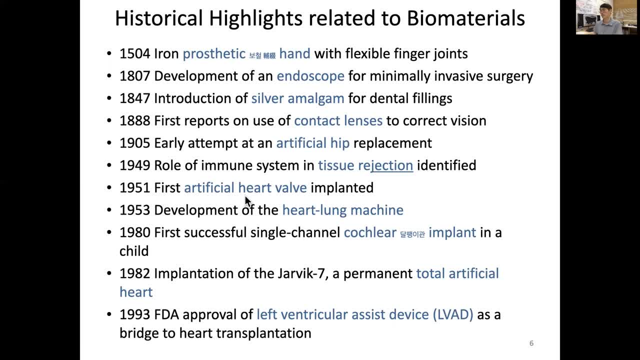 In 1951, the first artificial heart valve was implanted. This is a big story because this heart valve issue is very- it can be very fatal. So 1953, now developing heart lung machine for when there needs a heart, for heart transplantation during.